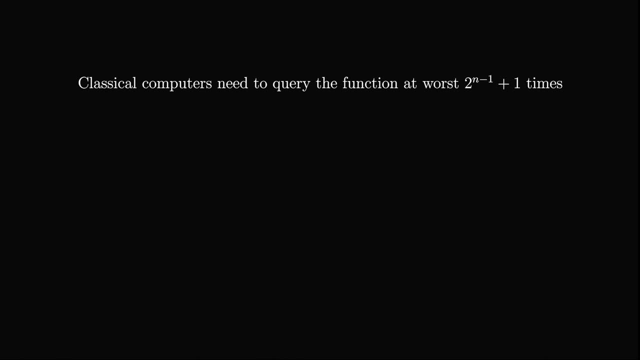 the function is balanced, This gives us a big O complexity of 2 to the power of n. With quantum computers, however, we only need one query of the function to find out if it's constant or balanced, giving us exponential speedup. 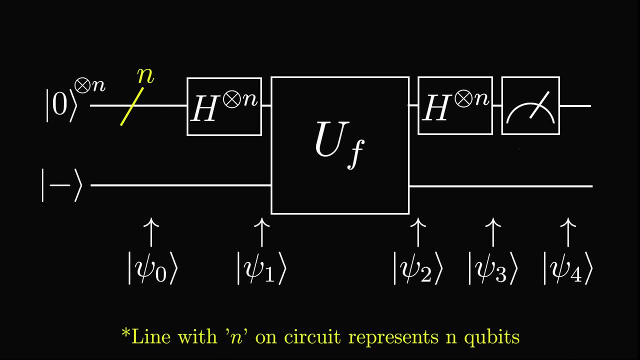 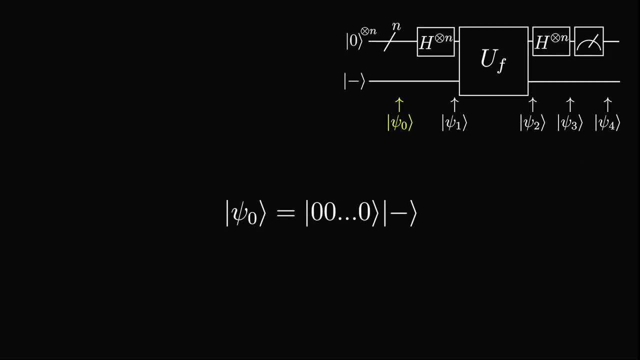 Here is a circuit for the algorithm. Let's label different parts of the algorithm with psi so that we can keep track of where we are in the circuit. Initially, the state is n zeros minus. We can rewrite the n zeros as this, Which means 0 tensed with itself n times, giving us this state. 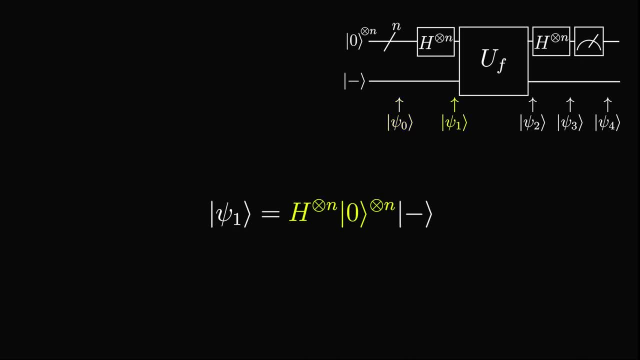 Then at psi, sub 1, we apply a Hadamard gate to each of the qubits in the first register. If we expand them out, then we have 1 over root, 2, 0 plus 1, tensed with 1 over root. 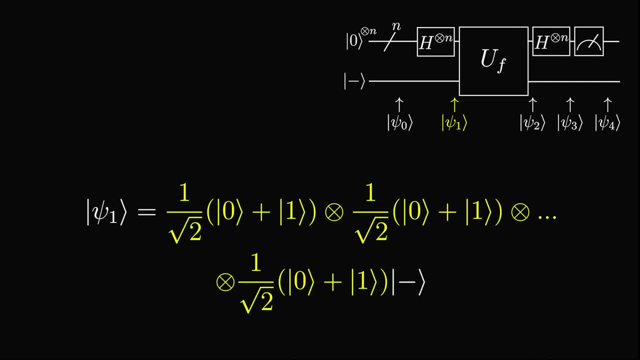 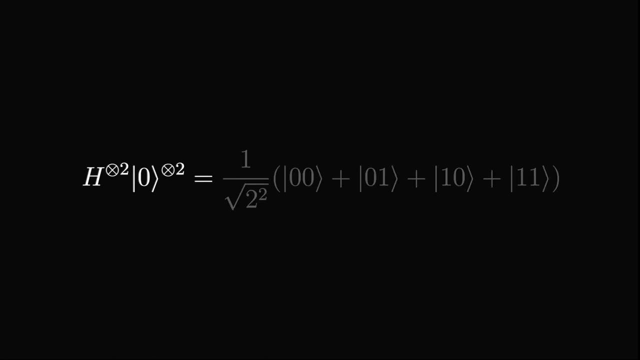 2,, 0 plus 1, and so on n times So that we can come up with an equation for this part of the state. let's try a different values event to find out how we can represent it. If we have n equals 2, so the plus plus state and we expand it out, it becomes 1 over root. 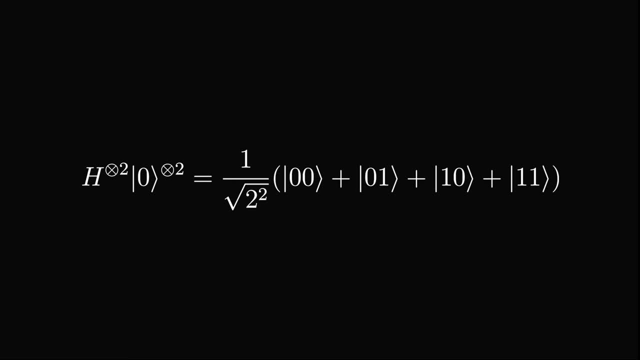 2 squared 0, 0 plus 0, 1 plus 1, 0 plus 1: 1.. If we have n equals 3, we get plus plus plus. If we once again expand this out, we get this: In the case where n equals 2, it equals 1 over 2 times the sum, over all possible x's. 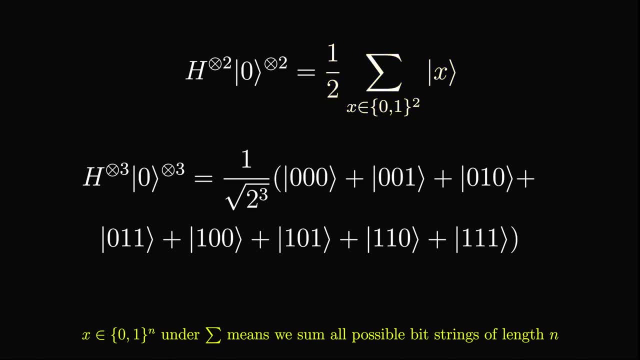 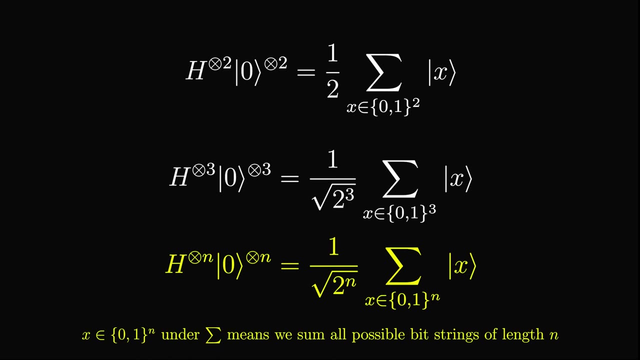 that are bitstrings of length 2, x. We can do the same thing for n equals 3.. Generalising these findings, we can see that applying Hadamards to a register of n zeros gives us the equation 1 over root 2 to the power of n times by the sum of all x's. that 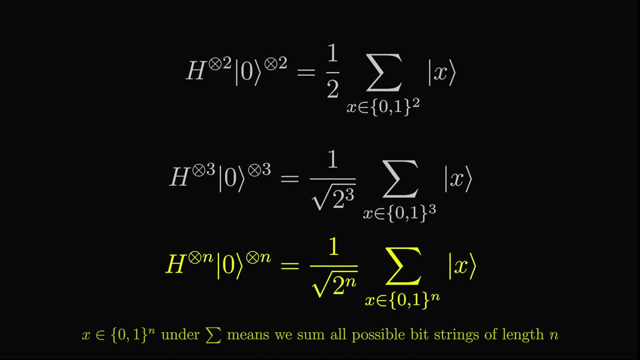 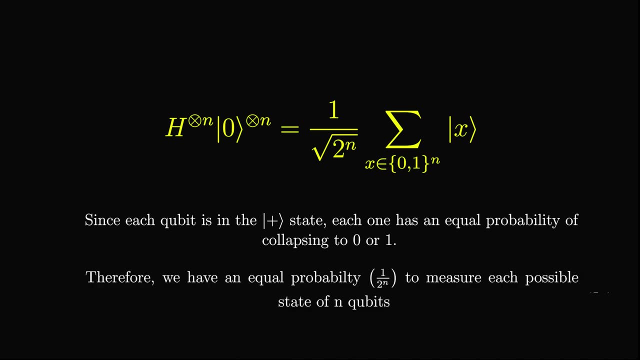 are bitstrings of length n, x. Intuitively this makes sense, since each qubit has an equal chance of being 0 or 1, so every possible combination of zeros and ones can occur and have an equal probability of occurring. 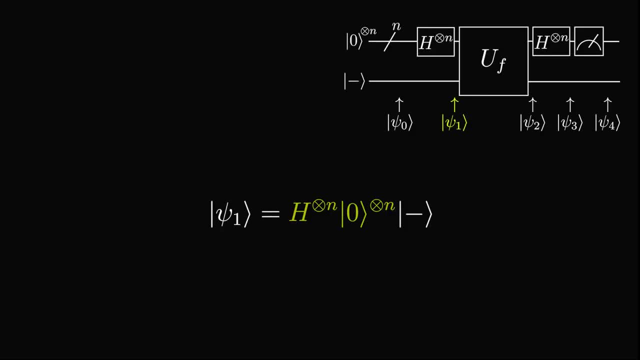 Thus we can represent psi 1 as 1 over the square root of 2, to the power of n times the sum over all x. where x is a bitstring of length, n, x At psi sub 2, we apply the oracle. 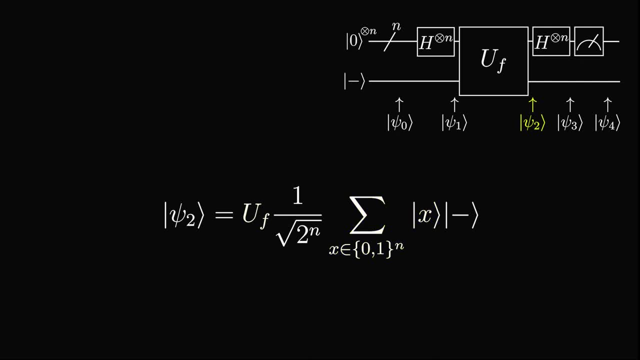 Since the input is in a superposition, the unitary matrix u of f acting as the function gets distributed into the sum. Now, if we look at each of the superposition states in the sum, Each of them has n bits as input and the minus state as output. 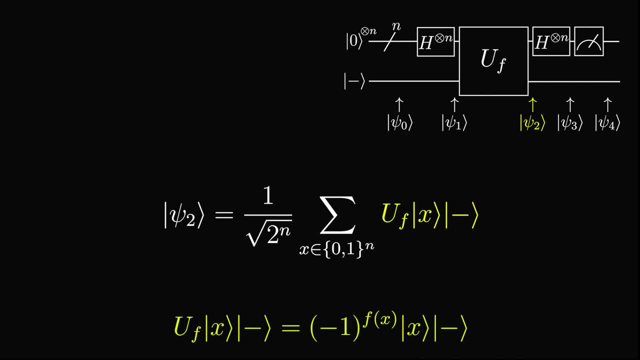 With that we can see that each state in the sum is in the phase oracle form. so when we apply the oracle we get phase kickback. Let's omit the minus qubit, since it is not needed for the rest of the algorithm. 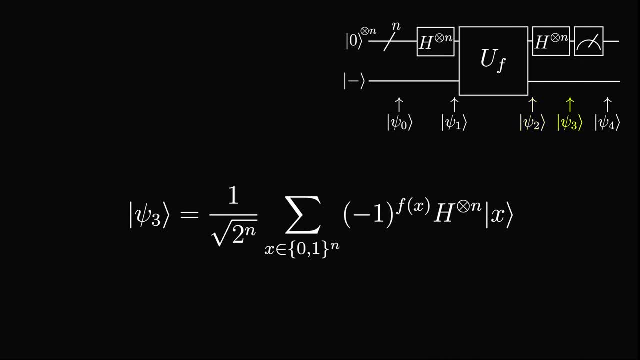 We now apply a Hadamard gate to each of the qubits. What this means is that for every bit in x- since x is a bitstring of length n- a Hadamard gate is applied. You might be thinking we could use the other formula that we used at the start of the algorithm. 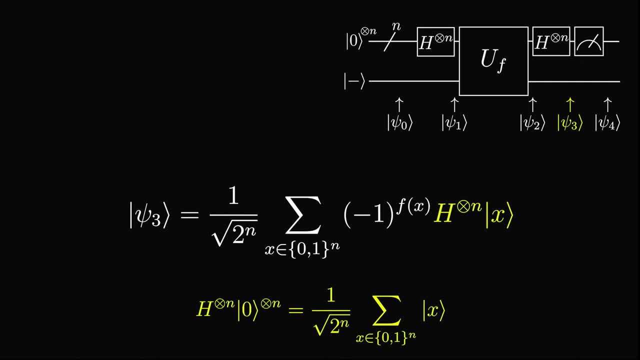 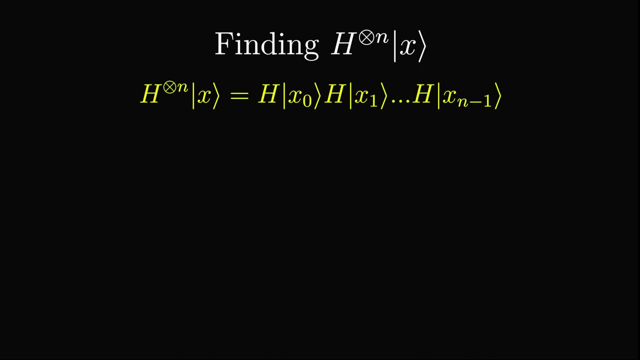 but that one is for Hadamards that are applied to all zeros. We don't know what x is. it could contain all zeros, both zeros and ones, or all ones. To find out how we can write this transformation, let's rewrite the Hadamard transform on. 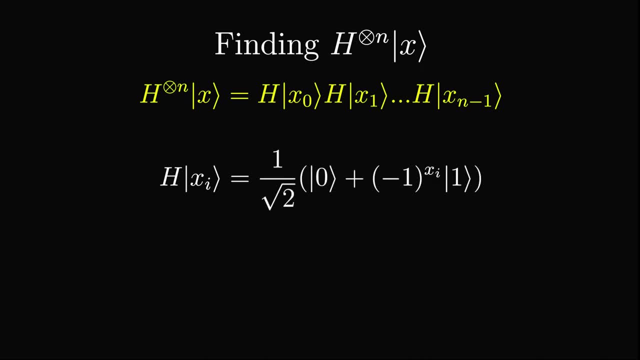 an arbitrary bit xi as 1 over root, 2, 0 plus negative 1 to the power of xi. 1. Since if xi is equal to 0, then it becomes 1 over root. 2. We can write the Hadamard transform on an arbitrary bit xi as 1 over root, 2, 0 plus. 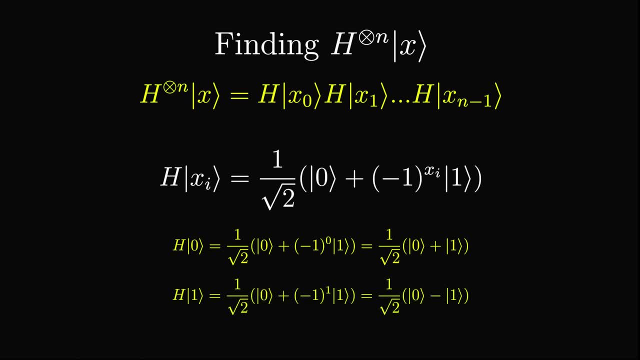 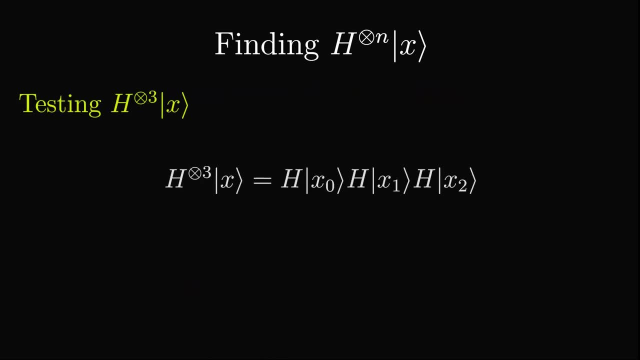 negative 1 to the power of xi, 1.. And if xi is equal to 1, then it becomes 1 over root, 2, 0 minus 1.. If we have the state x, which is a bitstring of length 3,, applying a Hadamard to each of. 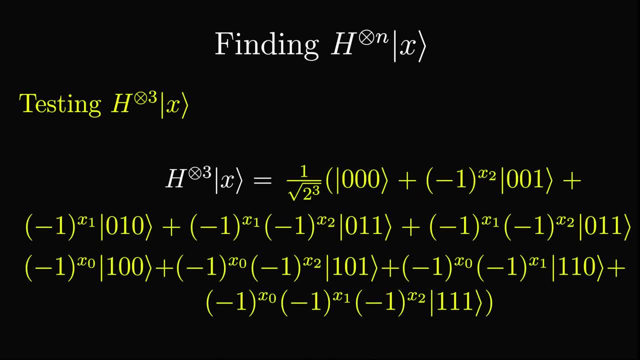 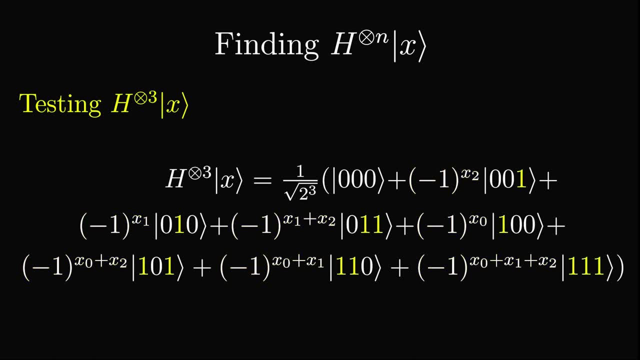 the two qubits, and expanding leaves us with this equation. Let's quickly clean up this equation by adding the exponents. As you can see, whenever there is a 1 in the state, negative 1 to the power of xi is times by that state. 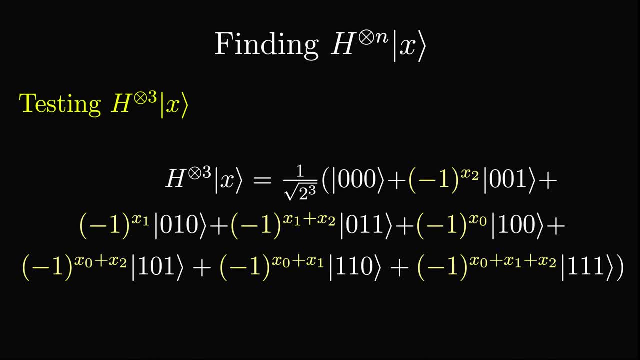 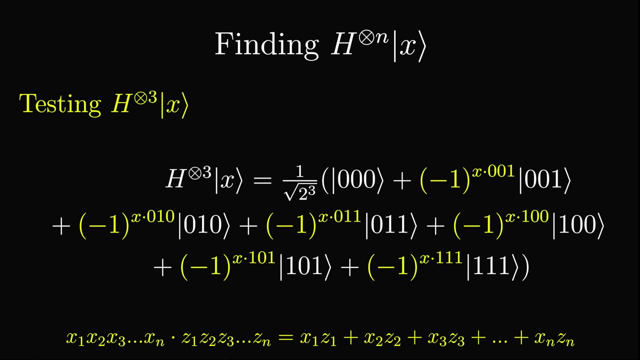 This is because x is a bit string. This is the position of the 1.. If we think about it, this is when both x and the new superposition coded by the Hadamards have a 1 in the same position. We can rewrite the exponents as the dot product of x with the superposition state. 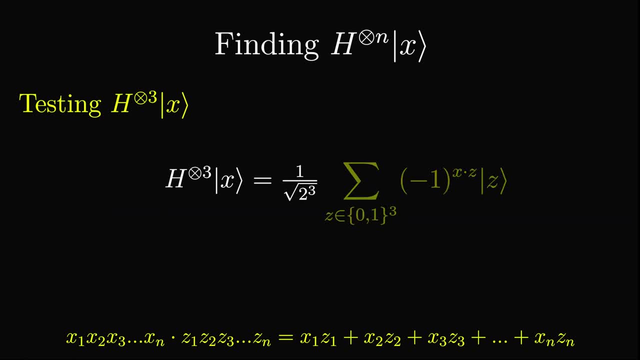 We can now rewrite the entire expression as the sum over all z's Negative 1 to the power of the dot product of x and z z. Intuitively this makes sense As at an arbitrary position i, both xi and zi must be 1 in order for a factor of negative. 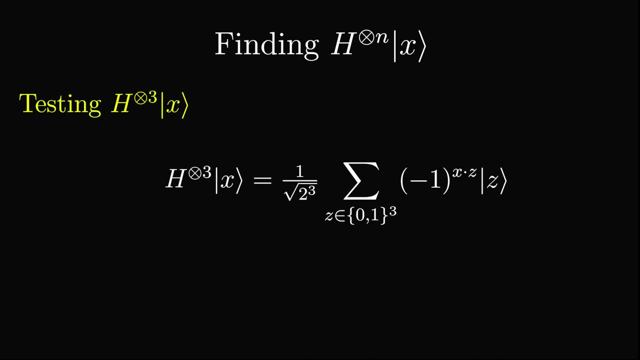 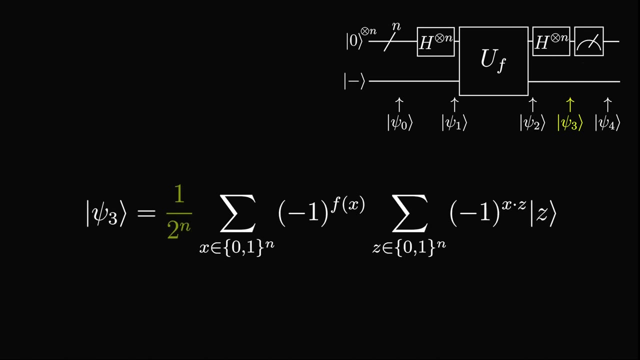 1 to be applied to that state, which matches up with the expansion we did earlier. This identity is very important and used in a lot of quantum algorithms. Now the qubits are in this state. Let's consider the amplitude of the all zeros state. 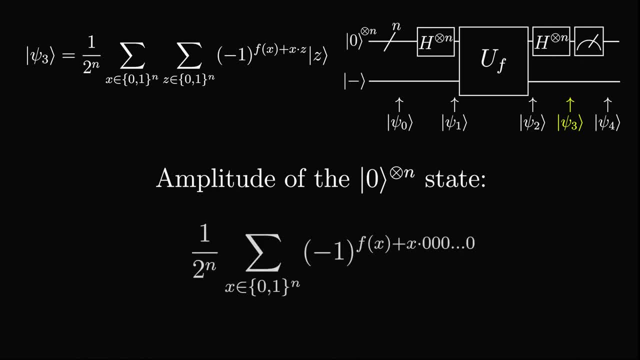 By expanding out the equation, we find that it is: 1 over 2 to the power of n times the sum over all x's negative 1 to the power of f of x plus the dot product of x with n zeros. 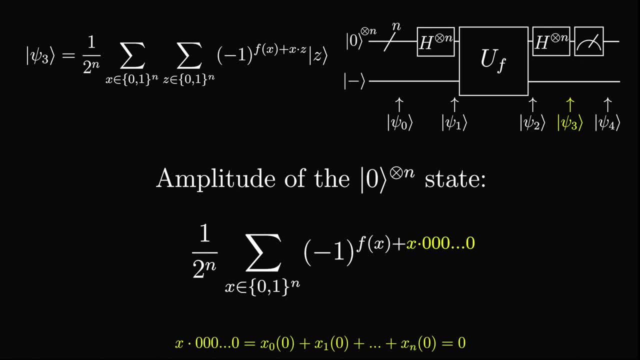 Since the dot product with all zeros equals zero, the exponent of negative 1 becomes f of x. Now let's consider two different scenarios. If f of x is constant, then for all x's f of x will always be the same value. 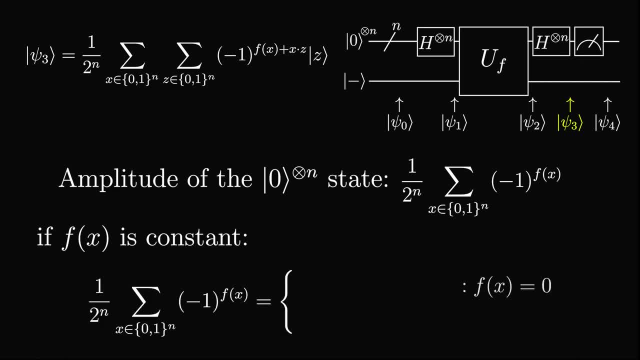 So the amplitude of the all zero state, if f of x is equal to zero, is 1 over 2 to the power of n times the sum over all x's that are bit strings of length, n, 1.. If we solve the sum, since there are 2, to the power of n possible combinations of x, 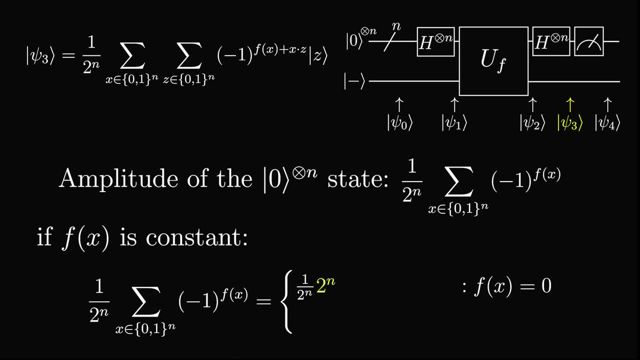 the sum becomes 2 to the power of n. The one over two to the power of n is negative: 1 to the power of n plus the dot product of to the power of n and 2 to the power of n. cancel, leaving us with just 1.. 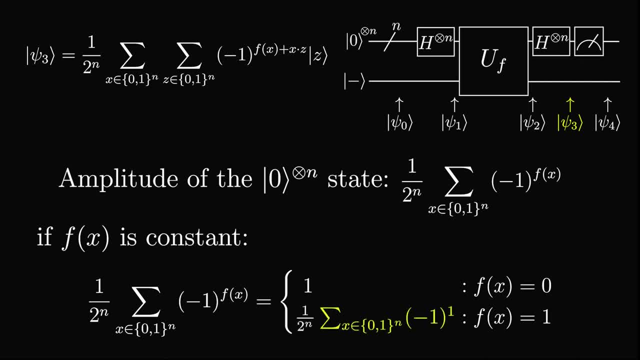 If f is equal to 1, on the other hand, we do the same thing, leaving us instead with 1 over 2 to the power of n times by negative 2 to the power of n. Simplifying it becomes negative 1.. 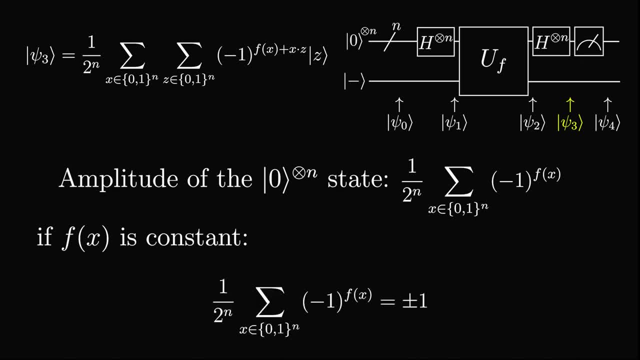 Combining these two. if the function is constant, then the amplitude of the all-zeros state is plus or minus 1.. This means that if the function is constant, the probability of measuring all zeros is 1.. On the other hand, if the function is balanced, then if we look at the sum half of the f